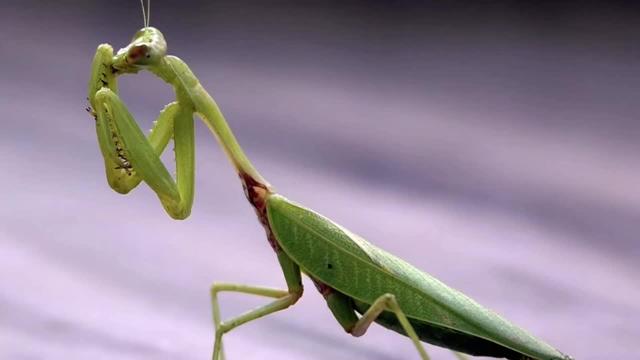 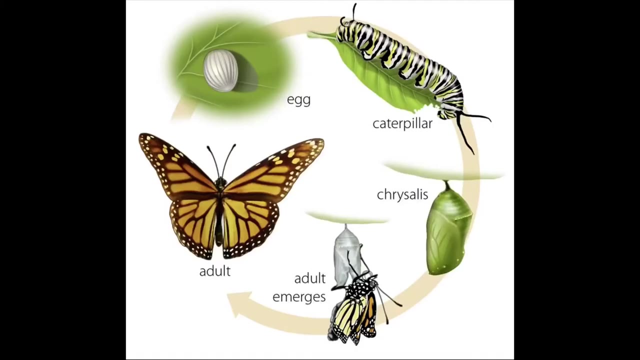 a butterfly. The name of the process in which a caterpillar changes or morphs into a butterfly is called metamorphosis. Some insects, like the butterfly, pass through four stages in their life cycles: Egg, larva, pupa and adult. Each stage looks completely different from the next: The young. 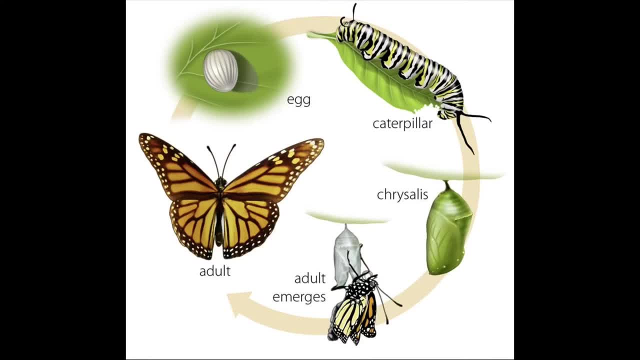 never resemble or look like their parents and almost always eat something entirely different. The female insect lays her eggs on a host plant or a plant on which another organism lives. When the eggs hatch, the larvae that emerge look like worms. The word larva is. 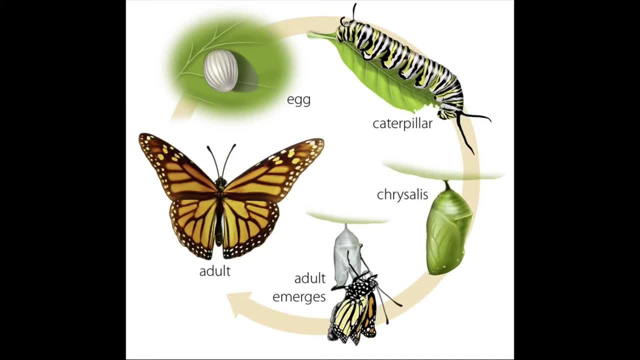 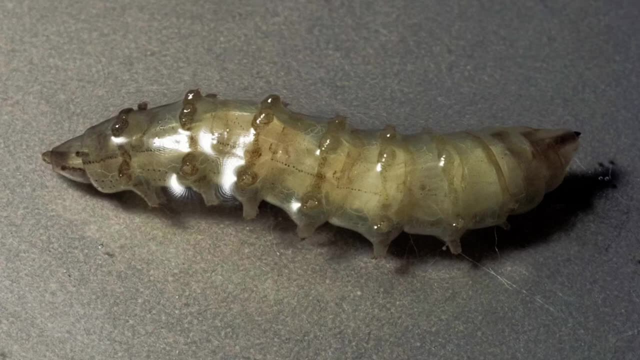 singular, meaning one, and the word larvae is plural, meaning more than one. Different names are given to different insects in this worm-like stage, and for the butterfly, the larva state is called a caterpillar, Fly larvae are called maggots, Beetle larvae are called grubs. 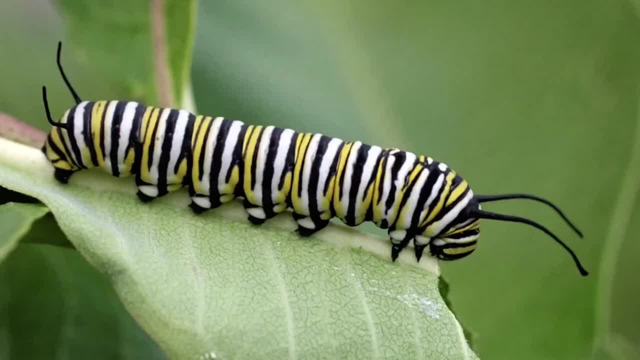 And the larvae of butterflies and moths, as you just heard, are called caterpillars. Larvae feed and grow as quickly as they can. They also molt or shed their hard exoskeletons many times as they grow, because the exoskeletons don't grow with them. In this way, insect larvae grow. 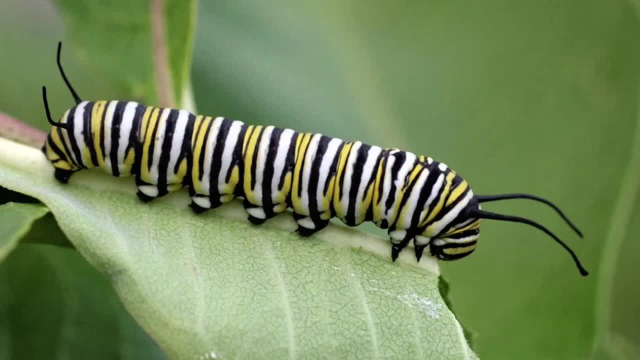 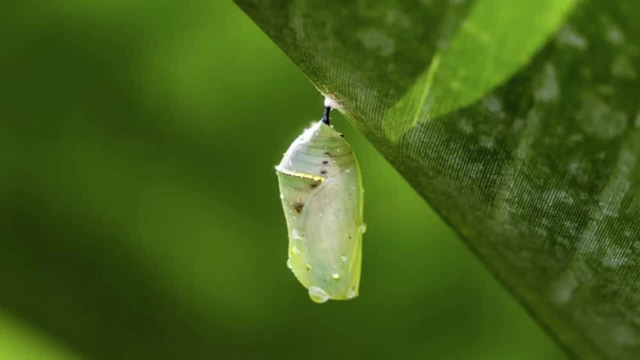 larger each time they molt until they are ready to change into adult insects. Once the larvae have eaten all that they can eat, they take a break. Sometimes people call this next stage a resting stage, but the larvae are hardly resting. A larva often spins a cocoon to protect. 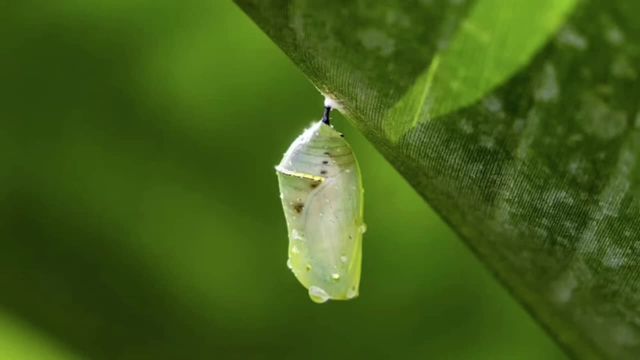 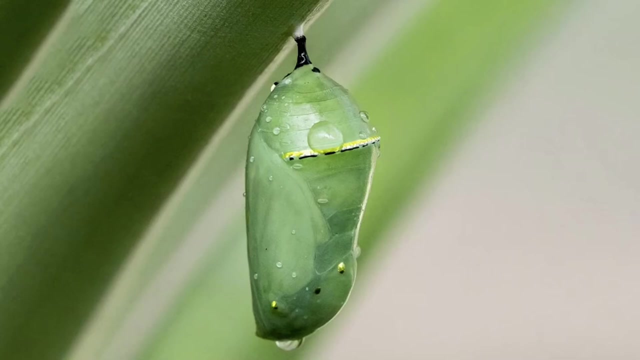 itself during the pupa stage, when it will remain quite still for several weeks Inside, this shell-like covering the pupa transforms or changes into something that looks altogether different than before. Some insects have a soft cocoon for the pupa stage and some, like the butterfly, have a 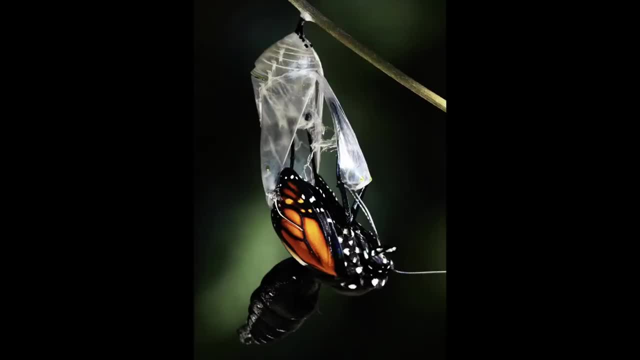 case called a chrysalis. If you have ever seen a butterfly emerge from its chrysalis, you know how extraordinary it is to watch the first flutter of its fully developed butterfly wings. Its wings were completely invisible before it disappeared into its seemingly magical chrysalis. It looks 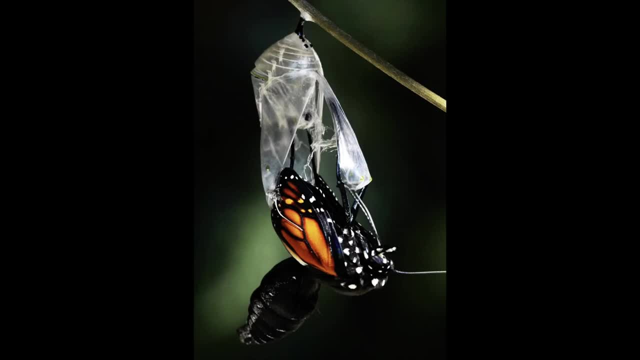 nothing like it did at any of its earlier stages. Scientists call this progression through four separate stages. If you have ever seen a butterfly emerge from its chrysalis, you know how extraordinary it is to watch the first flutter of its fully developed butterfly wings. Its wings were completely 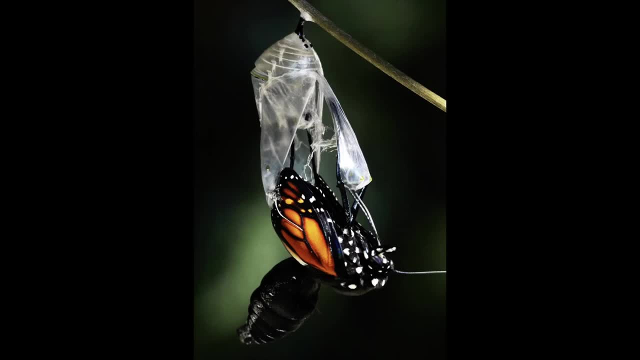 invisible before it disappeared into its seemingly magical chrysalis. It looks nothing like it did at any of its earlier stages. A complete metamorphosis, A progression, is a connected series of events. So a complete metamorphosis is a progression of events. I can't argue with that, can you? The change is indeed complete Butterflies. 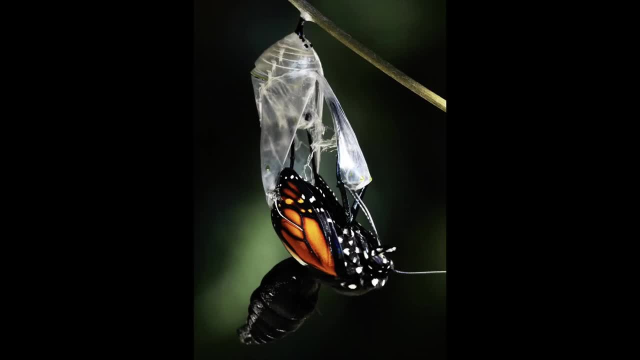 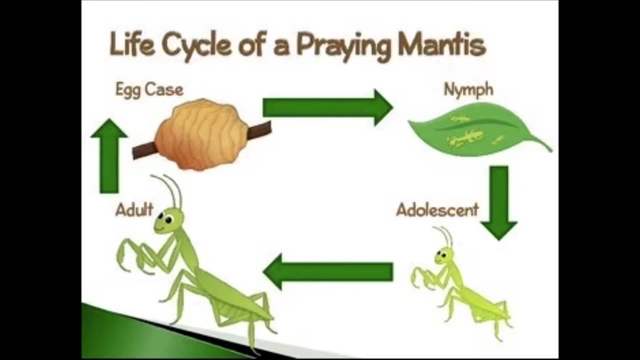 moths, beetles and flies all undergo a complete metamorphosis. Not all insects change so completely. Some insects, young like mine, are miniature or very small models of their parents after hatching. They do change, so they do experience. 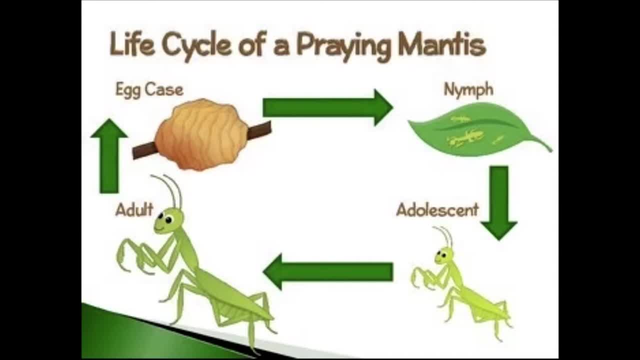 a metamorphosis, But because it is not a complete change, scientists call it an incomplete metamorphosis. Just like you, the young start off as a smaller version of what they will end up being, Just as you started off as a baby person and are slowly growing into an adult person. 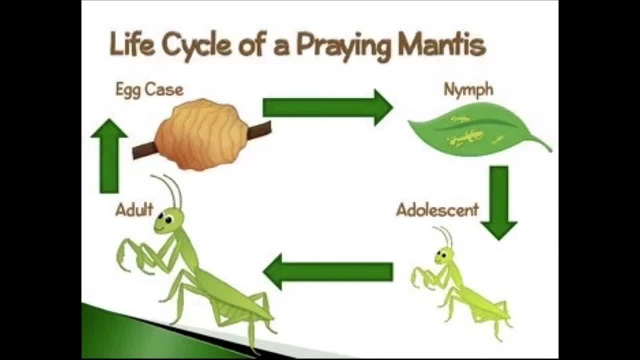 some young insects slowly grow and change. A praying mantis goes through three life stages: egg, nymph and adult. In autumn, the female mantis lays as many as 400 eggs inside an egg case attached to a plant. In spring, the eggs hatch. 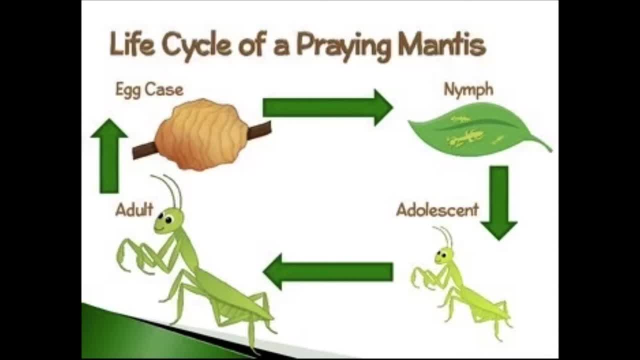 The tiny praying mantis babies emerge from the egg case. These brand new hatchlings, or nymphs, don't quite look like me, do they? A little later, the nymph resembles me more. The only thing it is missing is its wings. 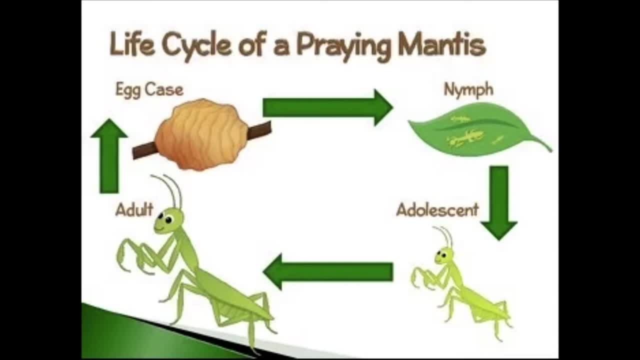 Even though you can't see them yet, there are tiny developing wing buds. These nymphs eat the same sorts of food as I do as an adult. praying mantis, Flies, aphids, moths and other insects, just smaller. 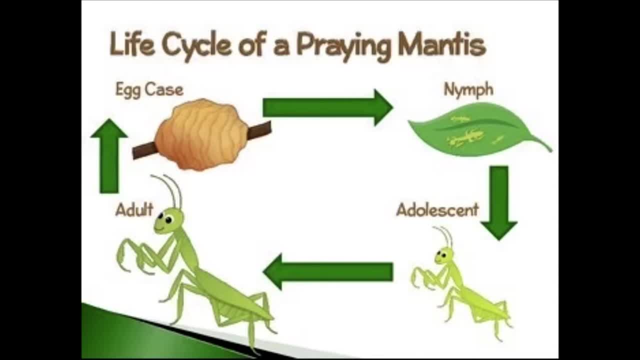 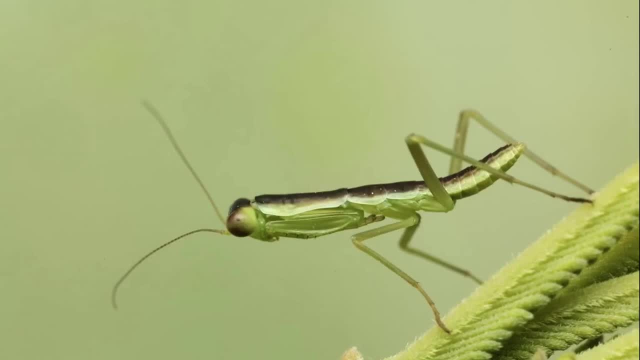 Let's take a close look at one of these nymphs. Can you tell at this stage that it is an insect? Can you feel it? Can you find its head? How many legs are on its thorax? Can you see how many pairs of wings it has? 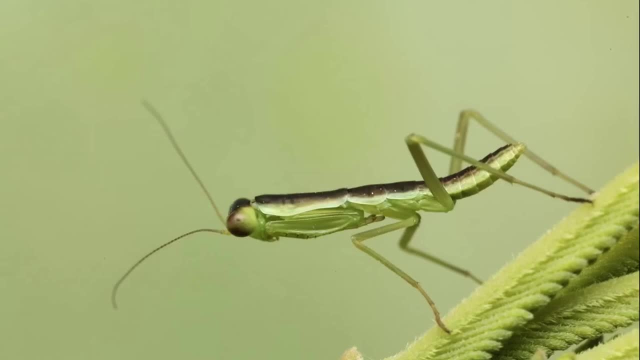 Is there a third section as well? What's that called? What is the outside skeleton of an insect called Right an exoskeleton? The baby insect or nymph is born with an exoskeleton, But these hard, non-living coverings do not grow with the growing praying mantis. 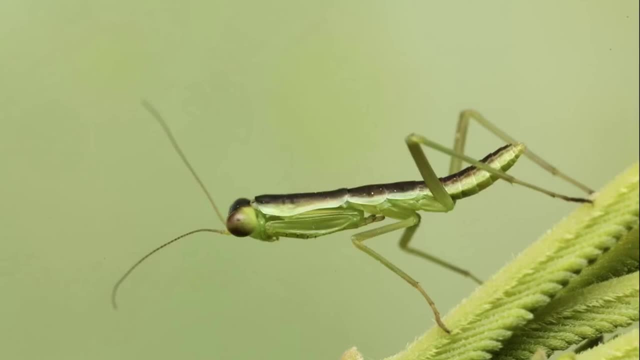 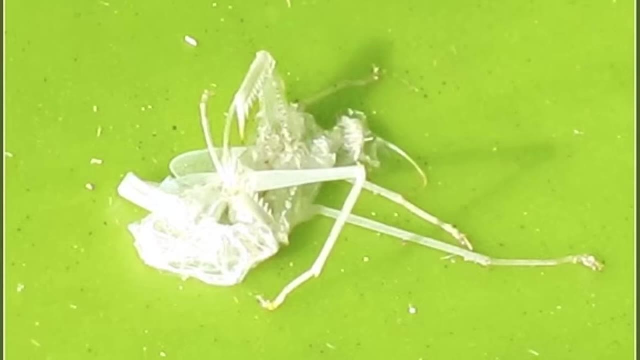 The nymph grows. its exoskeleton splits open. The nymph wriggles out to reveal softer skin that can stretch and expand before it hardens. It molds its exoskeleton again and again, growing a new one as many as ten times before it reaches adulthood. 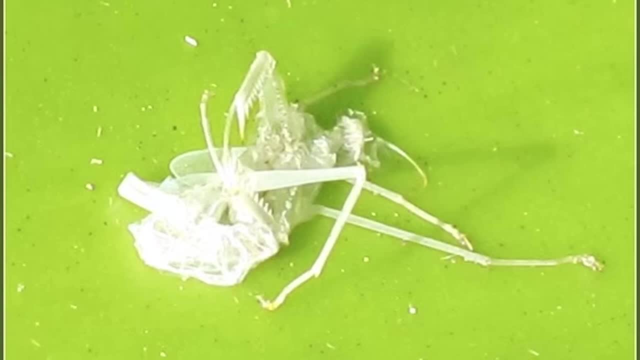 The nymph stage often lasts all summer, long After its final molt, each surviving praying mantis has a new one. After its final molt, each surviving praying mantis has a new one. After its final molt, each surviving praying mantis has a new one. 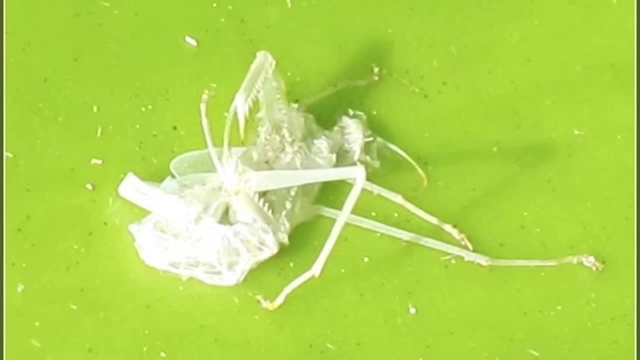 The mantis has a fully developed exoskeleton and full-grown wings, like mine. Grasshoppers, crickets and cockroaches belong to the group of insects that experience an incomplete metamorphosis similar to this one. An insect's life cycle is quite short compared to yours. In some cases, it takes only a few weeks. Scientists believe that this is one reason there are so many insects on the planet. They are forever breeding and need to reproduce. They are forever breeding and need to reproduce. They are forever breeding and need to reproduce. 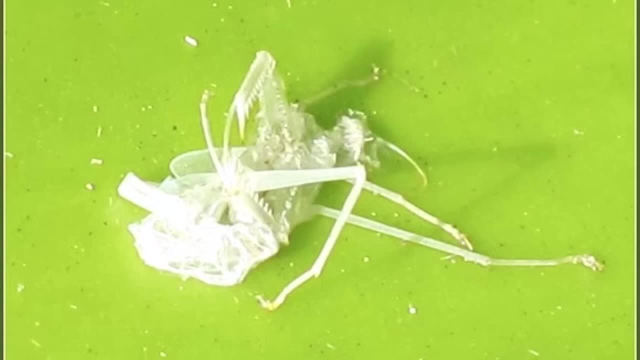 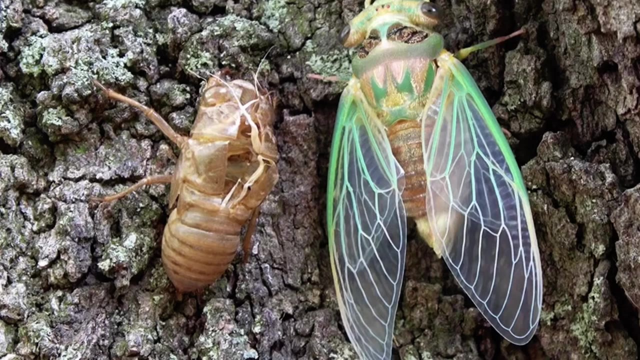 They reproduce rapidly because they have so many enemies. Not all insects, however, have short life cycles. The cicada looks a little like a grasshopper and is thought to have the longest life cycle of any insect, ranging from two to 17 years. 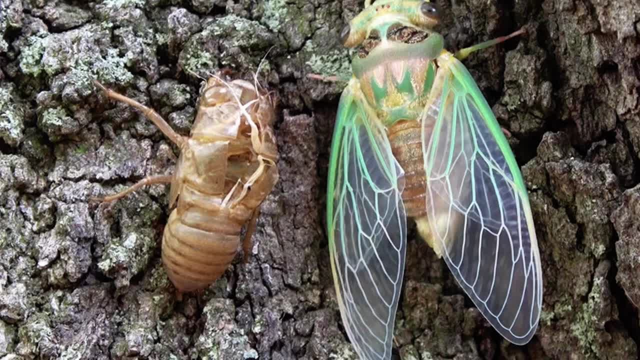 The adult cicada lays her eggs on twigs. When the eggs hatch, the nymphs fall to the ground and burrow under the soil searching for tree roots. They feed on the tree's sweet root sap. Cicadas undergo incomplete metamorphosis, so there is no.